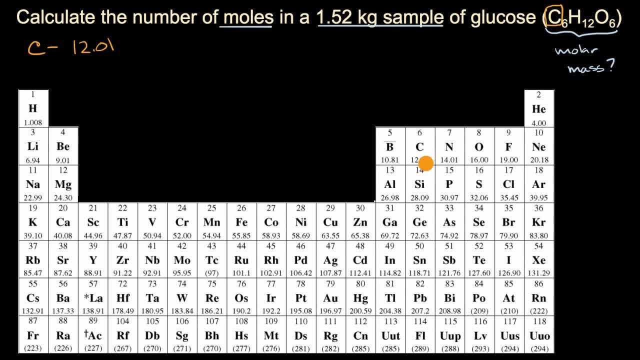 We've talked about in other videos. you could view this 12.01 as the relative atomic mass of a carbon atom, as the average atomic mass of a carbon atom or what's useful, and this is where Avogadro's number is valuable. 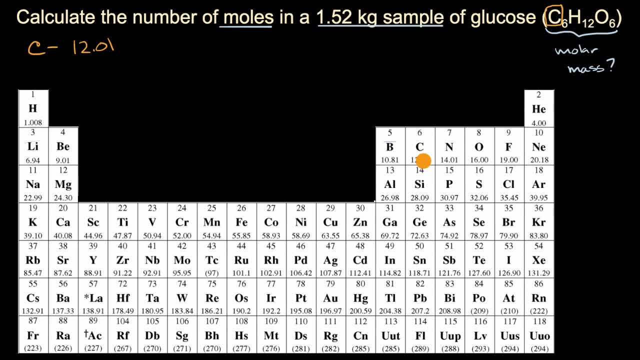 if you have Avogadro's number of carbons, it is going to have a mass of 12.01 grams. So carbon has a molar mass of 12.01 grams per mole. and now we can think about hydrogen in the same way. 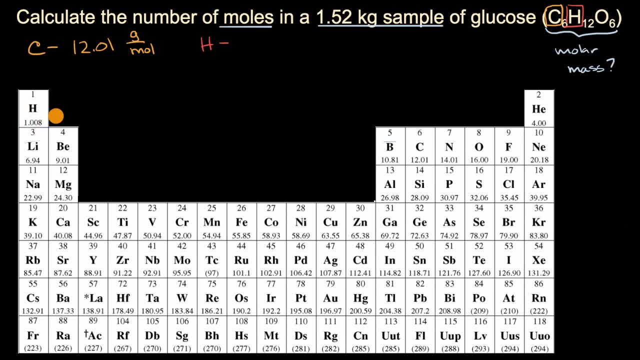 Hydrogen has a molar mass of 1.008 grams per mole- 008 grams per mole. And then, last but not least, we have oxygen here. Oxygen: we can see from our periodic table of elements: it has a molar mass of 16.00 grams per mole. 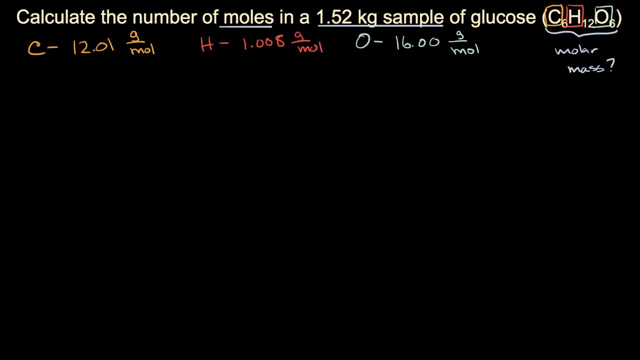 And so now we have all the information we need from our periodic table of elements. So the molar mass of glucose is going to be six times the molar mass of carbon, plus 12 times the molar mass of hydrogen, plus six times the molar mass of oxygen. 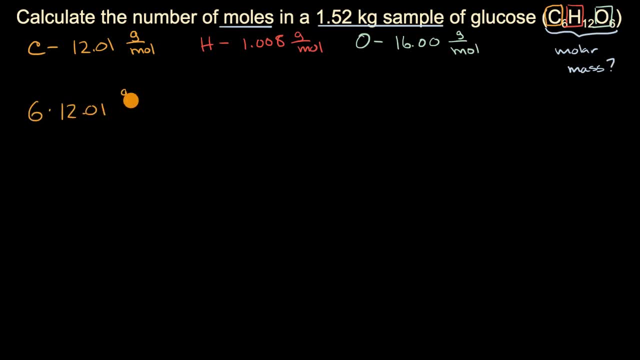 So it's going to be six times 12.01 grams per mole plus 12.01 grams per mole, So that's 12 times 1.008 grams per mole Plus. every molecule of glucose has six oxygens plus six times 16.00 grams per mole. 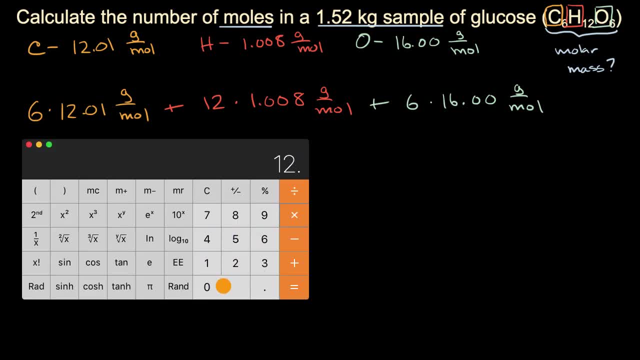 Six times 12.01, plus 12 times 1.008, plus 16.008 grams per mole. Six times 16 is equal to: and if we're thinking about significant figures here, the molar mass of hydrogen goes to the thousandths place. 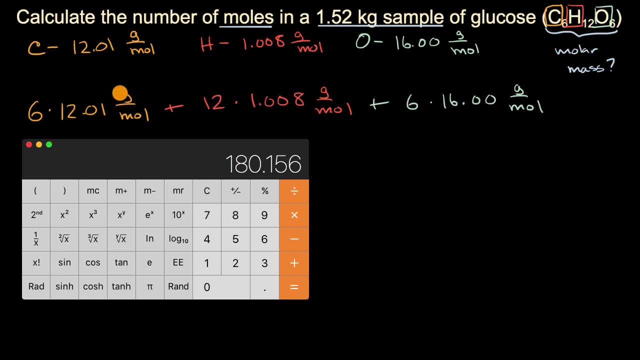 but we only go to the hundredths for carbon and for oxygen. We're adding all these up together, So it's going to be 180, point. I can only go to the hundredths place for significant figures. So 180.16.. 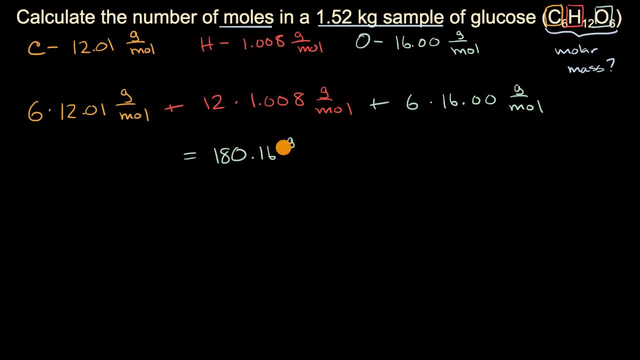 So that's equal to 180.16 grams per mole, And we could say grams of glucose C6H12O6 per mole of glucose C6H12O6, and then we can use this 1.52 kilograms to figure out how many moles we have. 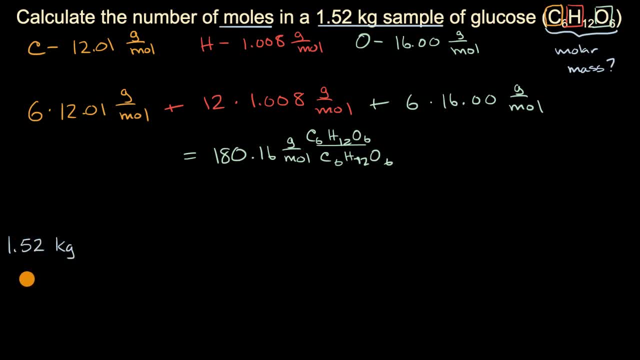 So if we start off with 1.52 kilograms of glucose, so that's C6H12O6,. well, first we can convert it to grams, because here the molar mass is given in terms of grams, So times we're going to want kilograms in the denominator. 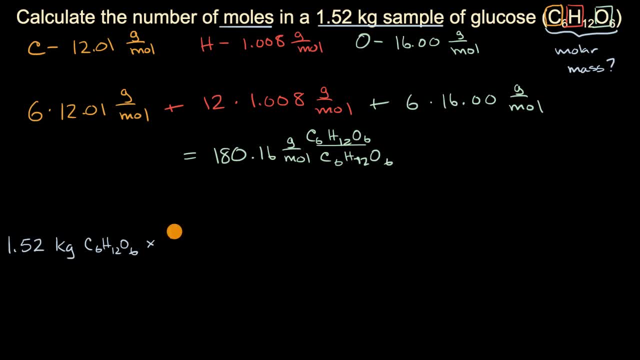 and grams in the numerator. So how many grams are there per kilogram? Well, we have 1,000 grams for every one kilogram. So when you multiply these two out, this is going to give you the number of grams we have of glucose, which would be 1,520. 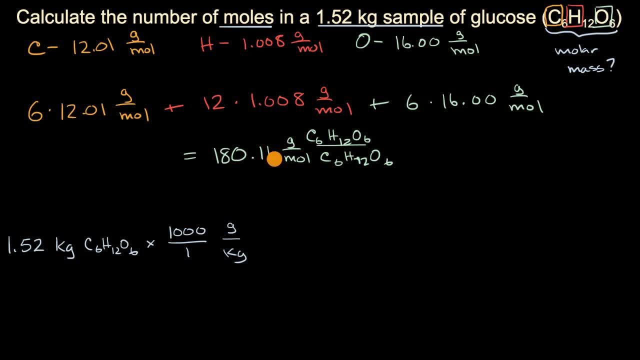 And if you have your mass in terms of grams, you can then divide by your molar mass, or you could view it as multiplying it by the moles per gram. And if you have your mass in terms of grams, you can then divide by your molar mass, or you could view it as multiplying it by the moles per kilogram. 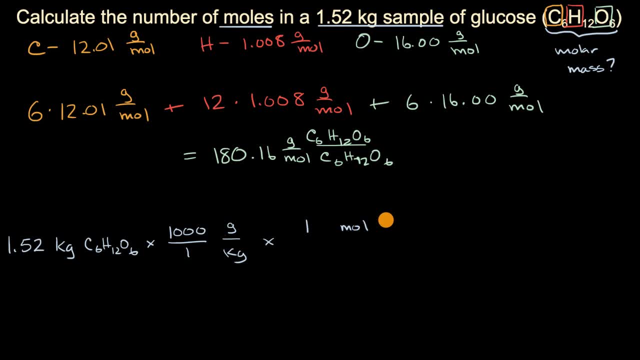 And if you have your mass in terms of grams, you can then divide by your molar mass, or you could view it as multiplying it by the moles per kilogram. So for every one mole of glucose, C6H12O6,. 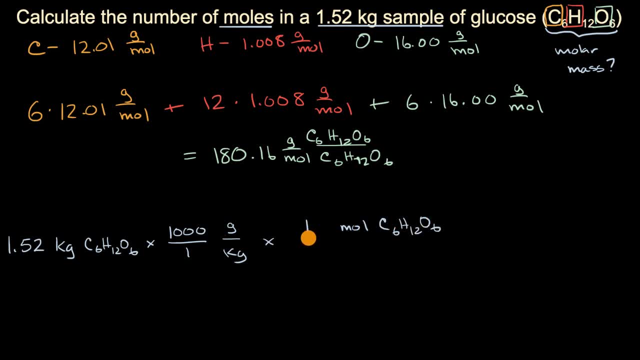 So, for every one mole of glucose C6H12O6,, we have 180.16 grams of glucose. we have 180.16 grams of glucose C6H12O6, and this is going to get us C6H12O6, and this is going to get us. 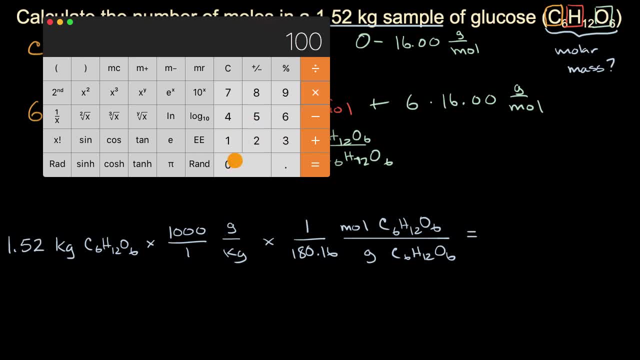 we get 1.52 times 1,000 is equal to. we get 1.52 times 1,000 is equal to. this is the number of grams of glucose. this is the number of grams of glucose, And then we're going to divide by 180.16,. 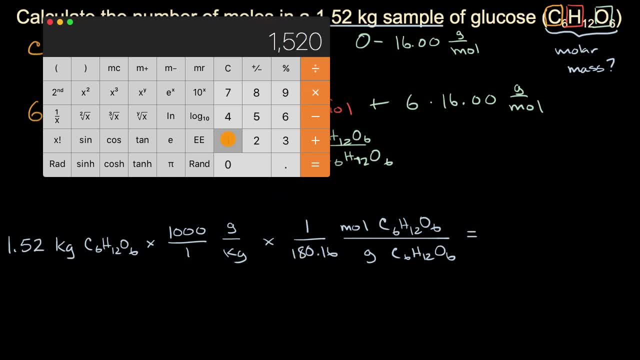 And then we're going to divide by 180.16,, divide by 180.16, gives us this number and let's see if we see significant figures. we have three significant figures here. we have five here, so we wanna round it. 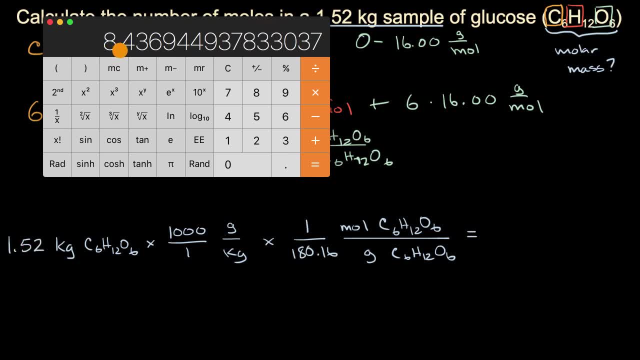 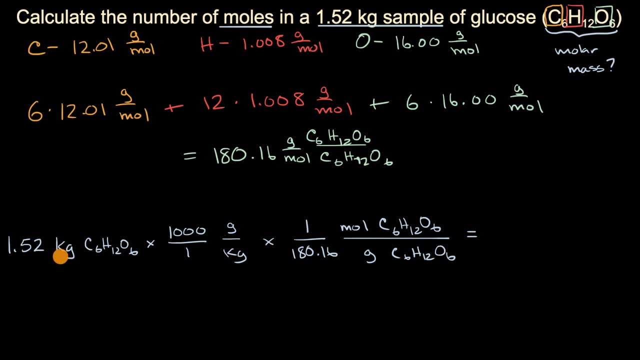 to three significant figures. So it will be 8.44 moles of glucose. So it will be 8.44 moles of glucose. So our, our kilograms cancel with our kilograms and then our grams of glucose cancel with our grams of glucose. 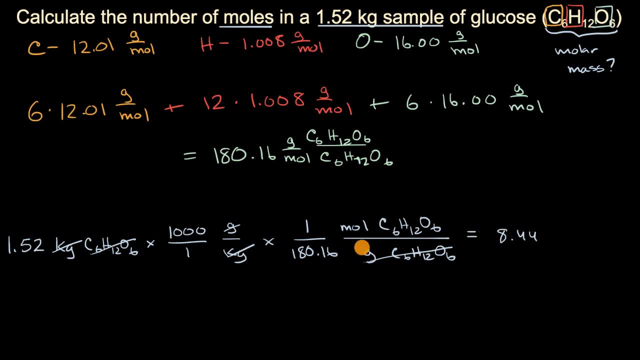 and we are left with 8.44 moles of glucose Moles of C6H12O6. And we are done. 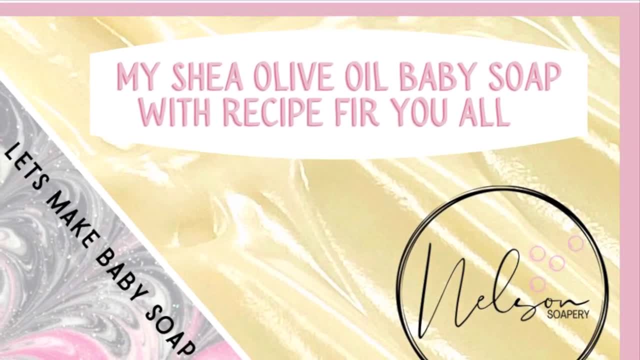 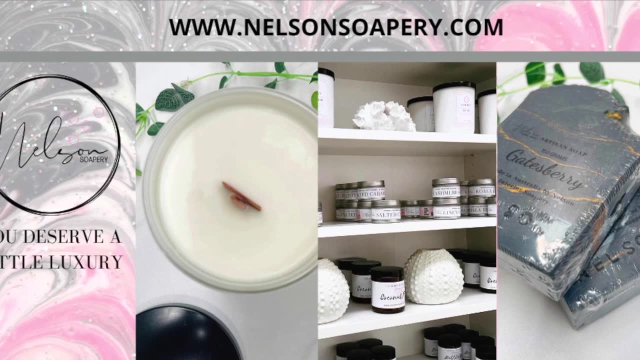 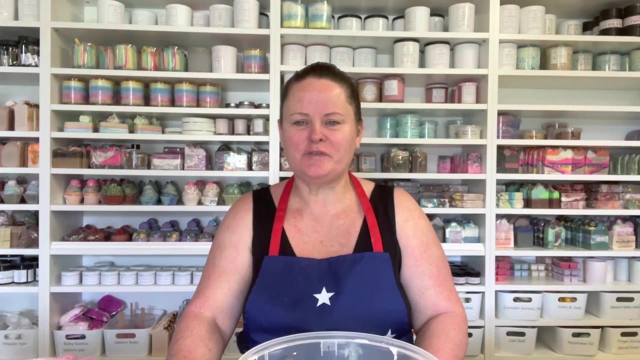 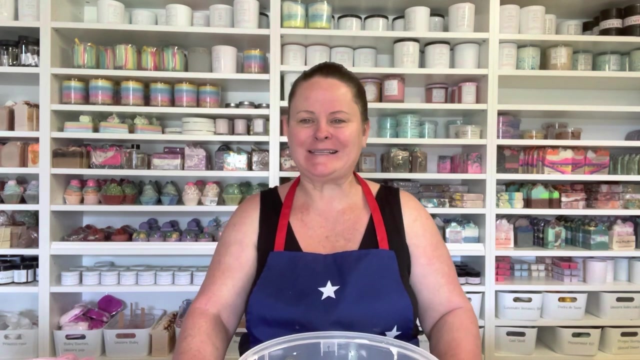 Hey everyone. it's Rhonda here from Nelson's Soapery. Today let's get into a video all about making beautiful baby soap. So to make baby soap, you don't need all the you know the massive ingredients that you would usually use. All we're going to be using is something beautiful. 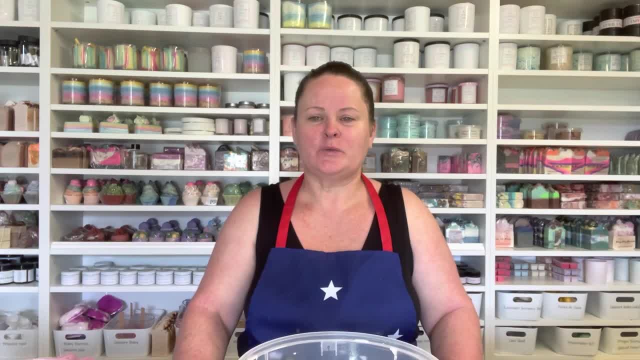 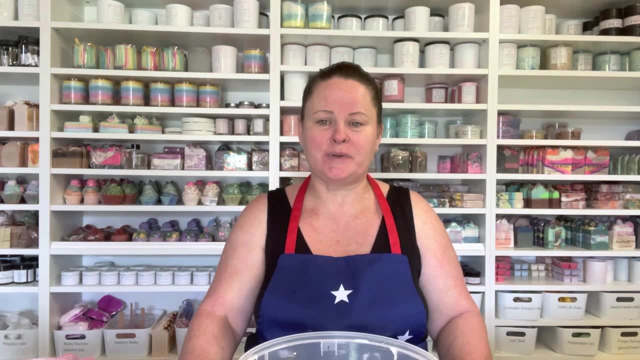 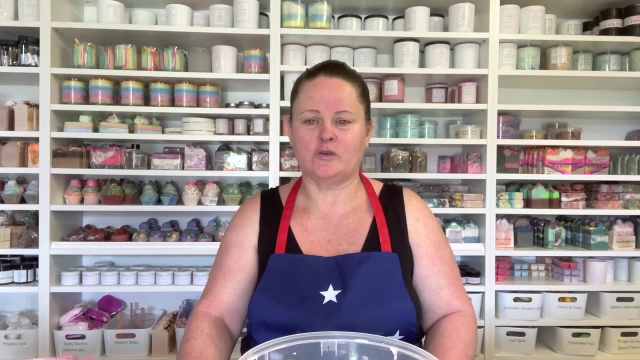 silky and doesn't have any cleansing at all. So when you put things like coconut oil into soap, coconut oil has a cleansing property, meaning a really big cleaning property, and of course, a tiny baby does not need that. They just need the beautiful things like shea butter or olive oil. 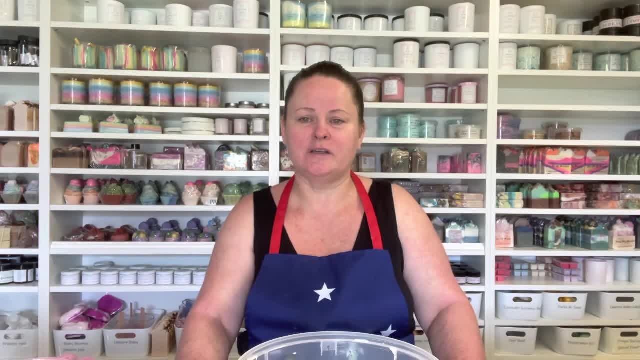 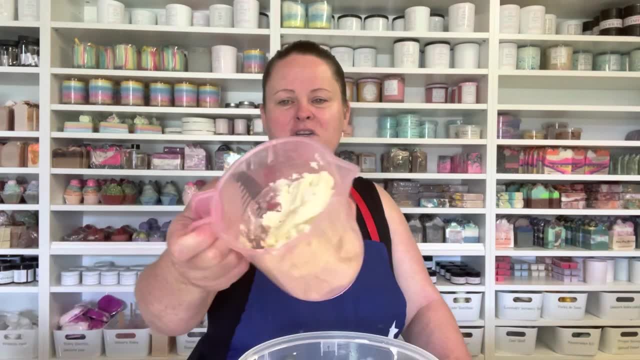 So everyone's different how they make these. You can make a pure olive oil baby soap, but I don't do that. My baby soap actually has a percentage of shea butter, which this is my gorgeous unrefined shea butter that I pop into it and, if you see, in my hand it's nice and squishy. 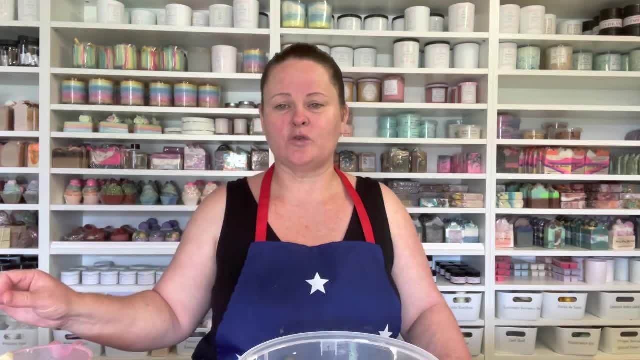 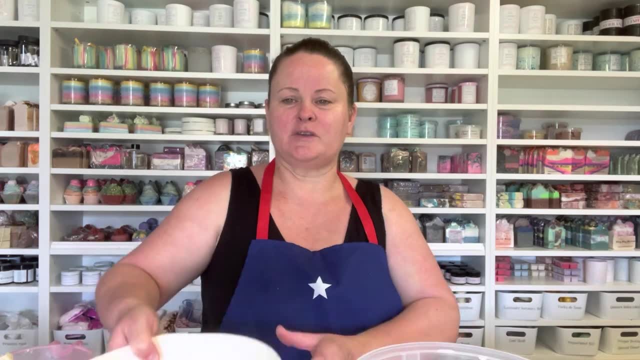 So you know, it's definitely really really soft and gorgeous and it will just add kind of that layer of a barrier to protect the baby skin. And then, of course, I have some absolutely beautiful olive oil in here, So it's going to be a massive base of olive oil. Of course, you do need the lye. 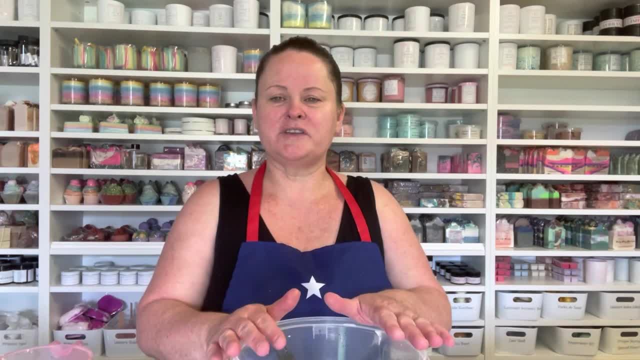 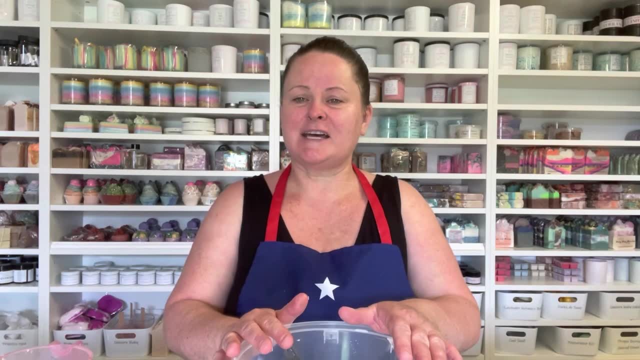 and everything to make soap, but you don't need to worry, It's more than safe to use for a baby. My little grandbabies do. I make it for them as well. So anyway, let's get started and we'll make a batch of this.